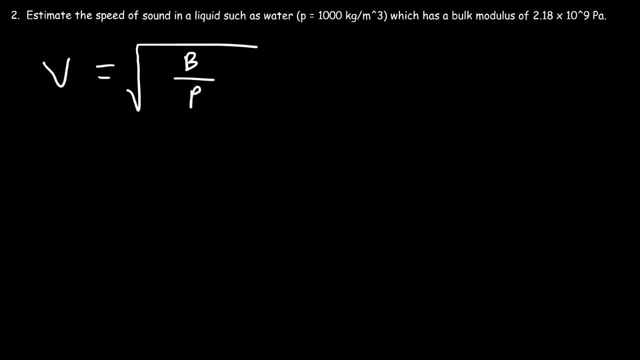 is going to be the bulk modulus divided by the density, And so we have the bulk modulus and the density of water is 1,000 kilograms per cubic meter, And so this is going to be about 1476 meters per second. So that's an estimate. 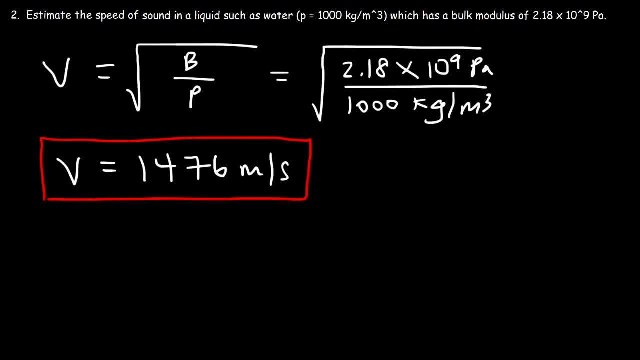 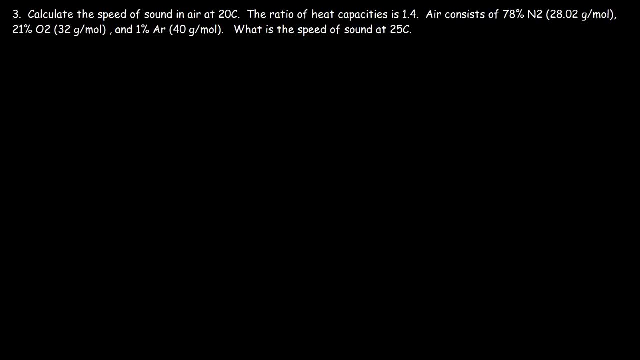 So that's the speed of sound in water. Number three: calculate the speed of sound in air at 20 degrees Celsius. Number three: calculate the speed of sound in air at 20 degrees Celsius. The ratio of heat capacities is 1.4.. Air consists of 78 percent nitrogen. 21. 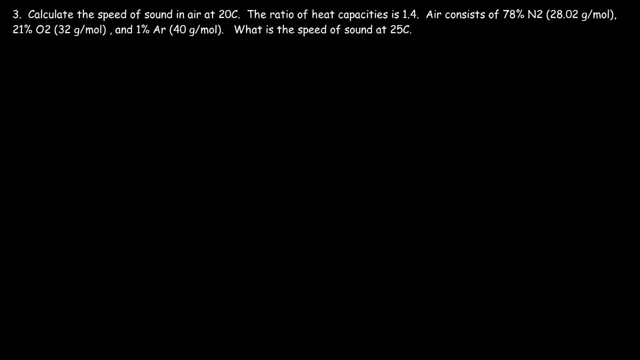 percent oxygen, 1 percent argon, and we're given the molar mass of these gases. What is the speed of sound? at 25 as well, And there's supposed to be a question mark here, But let's focus on the first temperature, at 20.. So the formula that we 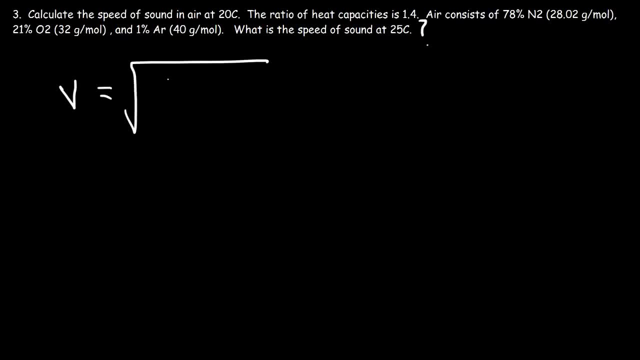 need is this equation? It's equal to gamma times R, which is the gas constant times the Kelvin temperature divided by the average molar mass of air. So let's calculate this value. first. We have gamma, the ratio of heat capacities, That's. 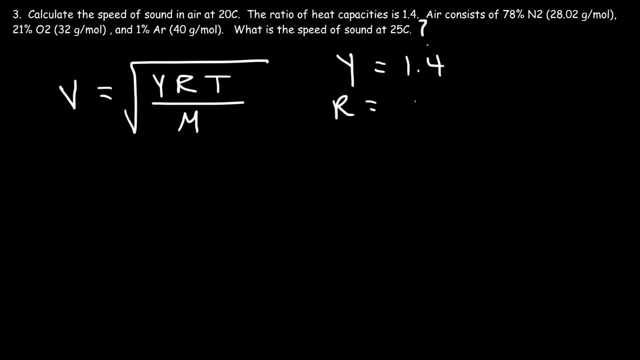 1.4.. And R is another constant. That's 8.3145 joules per mole per Kelvin. So the temperature has to be in Kelvin. So to convert Celsius to Kelvin, add 273 to it. So 20 plus 273 is 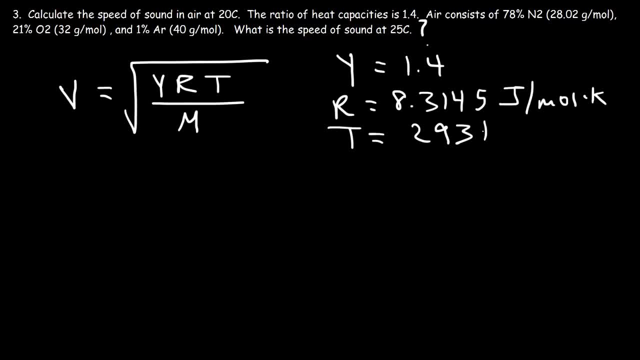 293 Kelvin. The last thing we need is the average molar mass, So the molar mass of nitrogen gas. if you look at the periodic table, it's going to be 14.01 times 2 or 28.02.. And air is 79 percent. I mean 78 percent nitrogen. So we need to multiply that by 0.78. 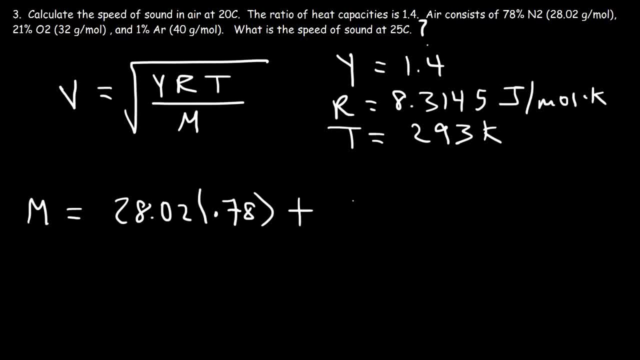 to calculate the average molar mass of air. Oxygen has a molar mass of 32,, and air is about 21 percent oxygen And argon is, or has a molar mass of 40,, and air consists approximately about one percent of argan. 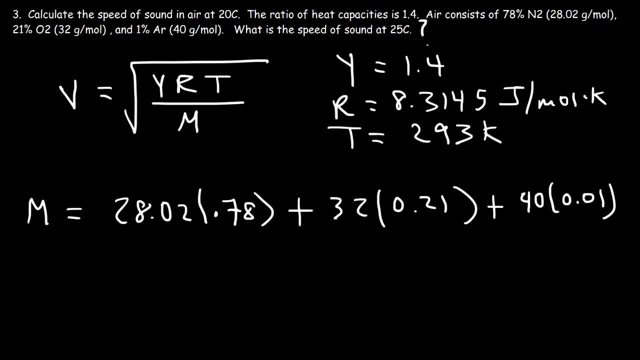 So let's put these numbers together in the calculator. Let's see what we get. So the average molar mass is about 29 grams per mole. Now we need this answer in kilograms per mole. So let's convert grams to kilograms. One kilogram is equal to a thousand. 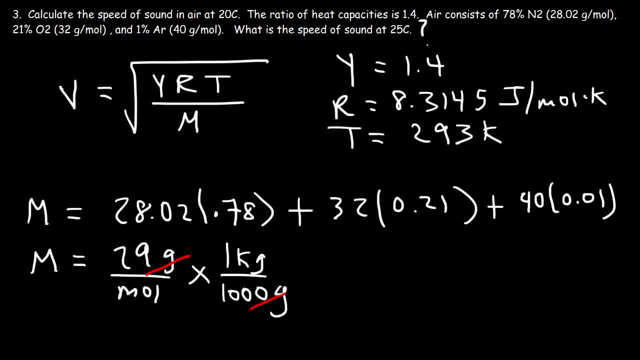 grams. So we need to divide this number by a thousand, So this is going to be 0.029 kilograms per mole. So now we have everything that we need to plug into this formula. So it's going to be 1.4 times 8.3145, multiplied by a Kelvin. 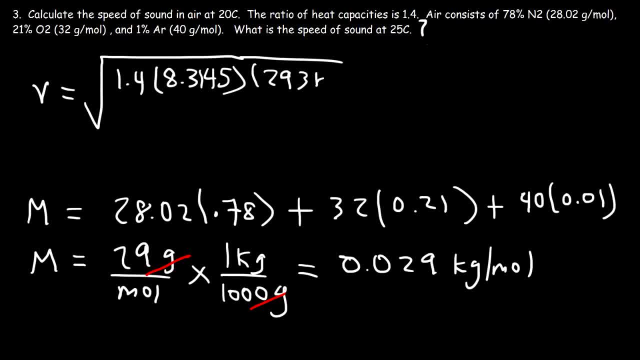 temperature of 293 divided by the molar mass, which is in kilograms per mole. So this works out to be 343 meters per second. So that's the speed of sound in air at 20 degrees Celsius. Now let's find out what it is at 25 degrees Celsius. 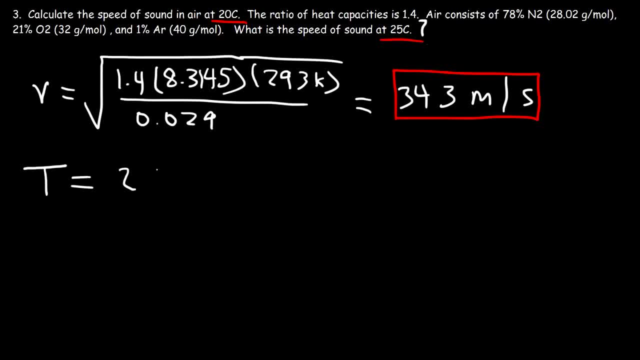 So first we got to find the Kelvin temperature. So it's 25 plus 273.. So it's a little bit higher. It's going to be 298 Kelvin. So everything's going to be the same except the new temperature. So let's go ahead and plug this in. 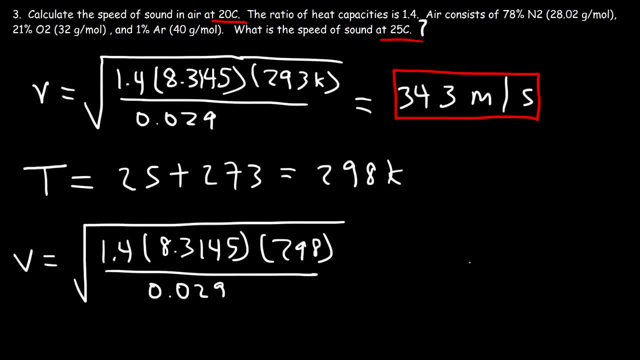 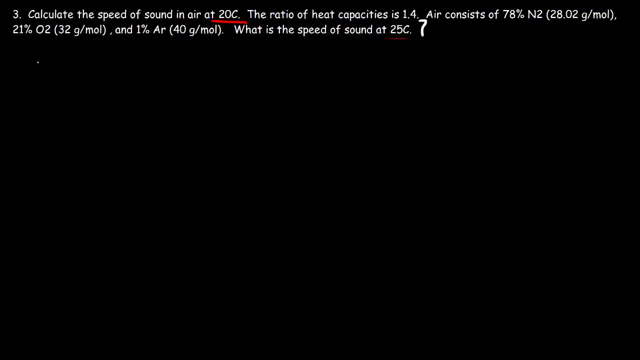 So this is going to be 346 meters per second. So, as we could see, as the temperature goes up, the speed of sound increases in air. Now there's another simple equation that relates temperature and the speed of sound, And here it is. 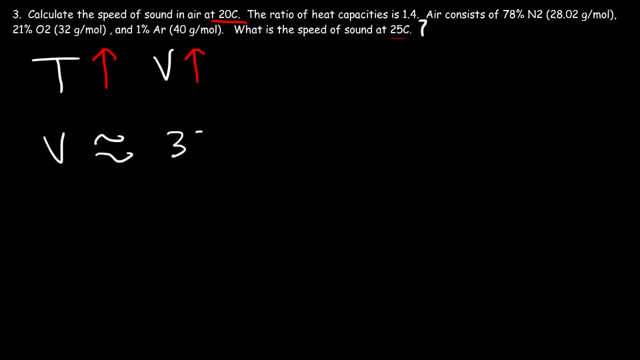 The speed of sound in air is approximately 331 meters per second plus 0.6 times T, where T is in Celsius. So, at 20 degrees Celsius, it's approximately 331 plus 0.6 times 20.. And so this will give you 343 meters per second. 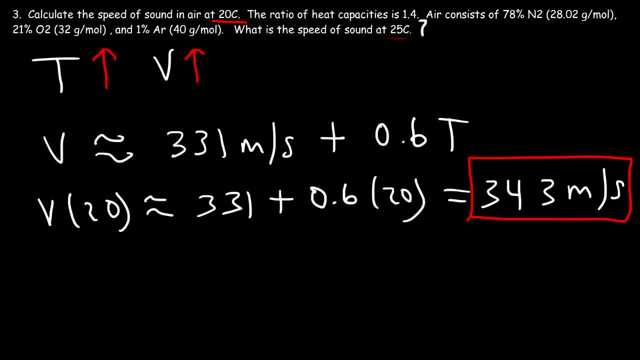